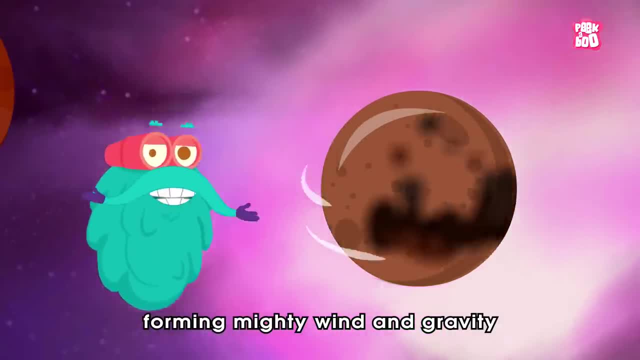 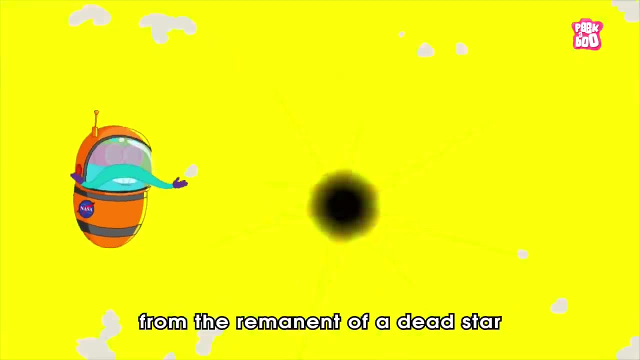 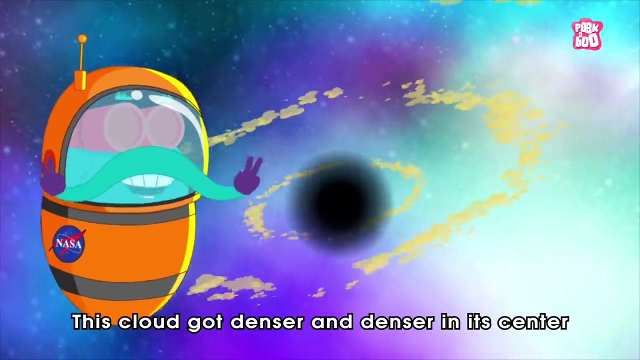 Everything started to spin, forming mighty wind and gravity, And over time one such gravitational force from the remnant of a dead star started pulling the giant dirty gas cloud. This cloud got denser and denser in its center and formed an accretion disk. 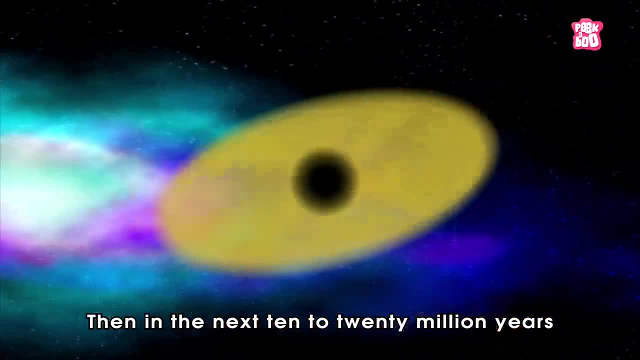 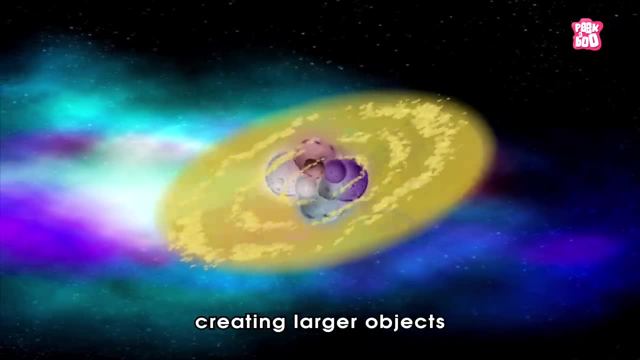 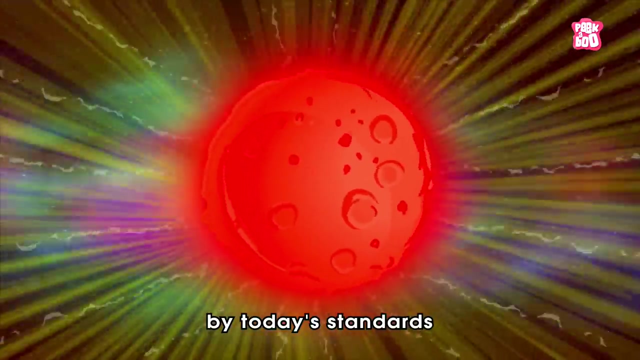 Then, in the next 10 to 20 million years, other small particles of dust, rock and gas started sticking together, Creating larger objects, Until it became a sphere and large enough to be called a planet by today's standard And young earth was formed. 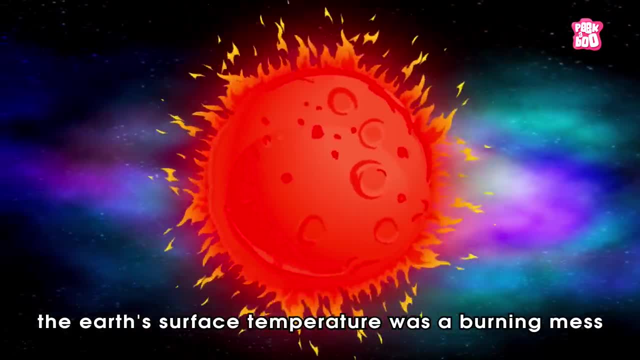 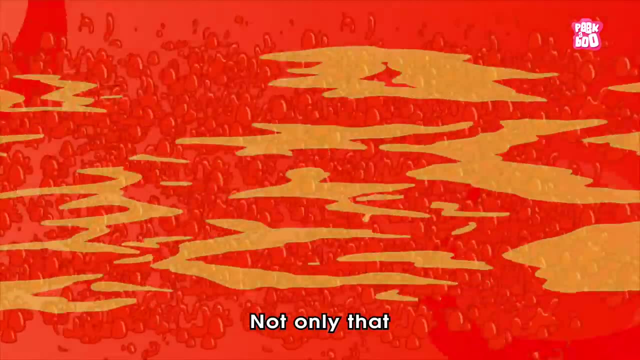 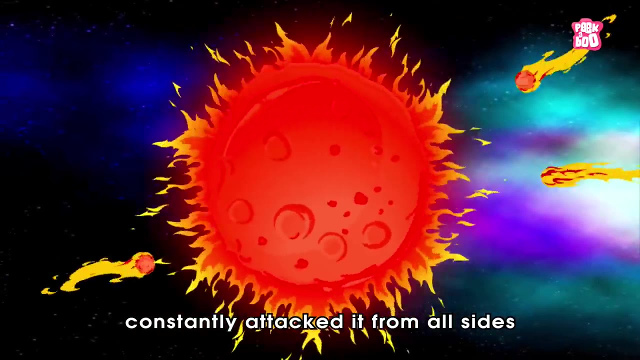 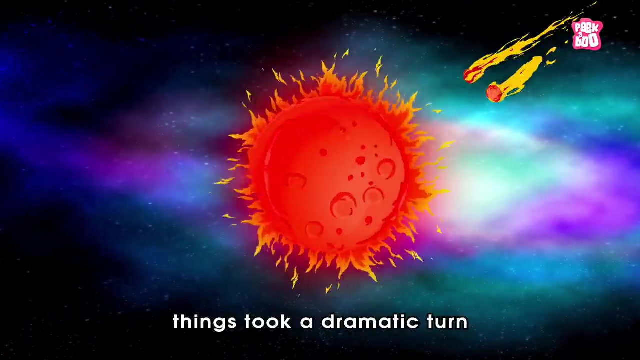 At this point, the earth's surface temperature was a burning mess, With seas of lava and a poisonous atmosphere. Not only that, various comets, asteroids and other cosmic elements constantly attacked it from all sides, Making it boil more and more, But soon things took a dramatic turn and the cosmic attack reduced. 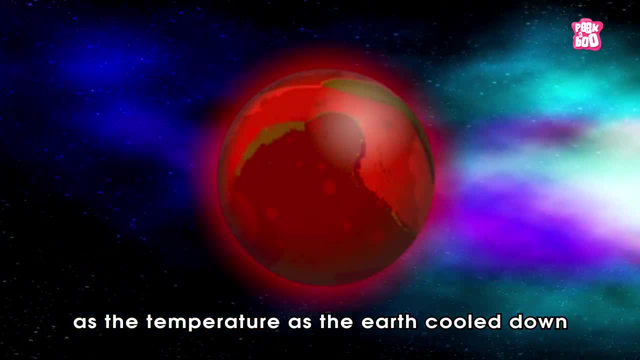 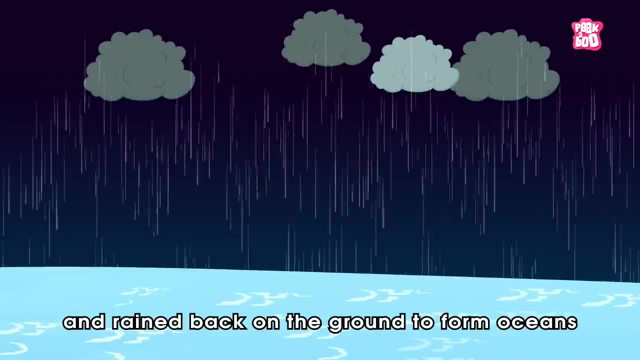 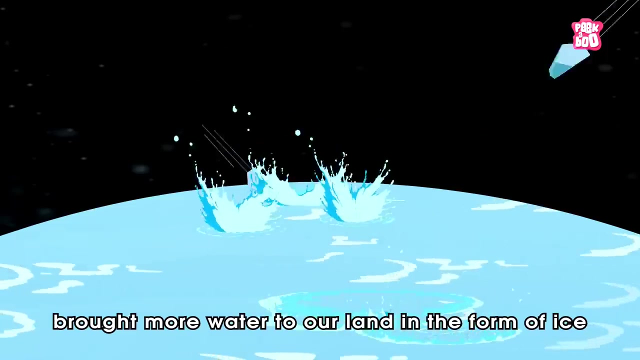 And so, as the temperature of the earth cooled down, Water from the inside of the earth rose to the surface, Formed steam and rained back on the ground to form oceans. Even other meteors brought more water to our land in the form of ice. 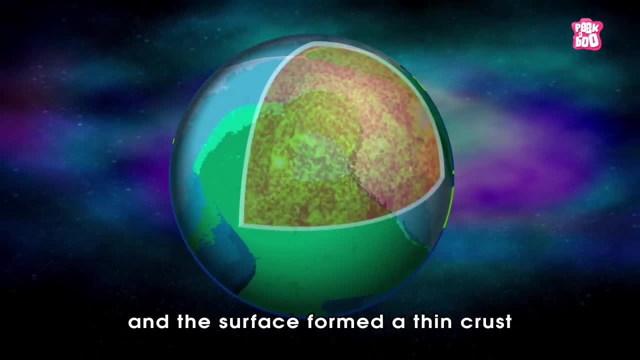 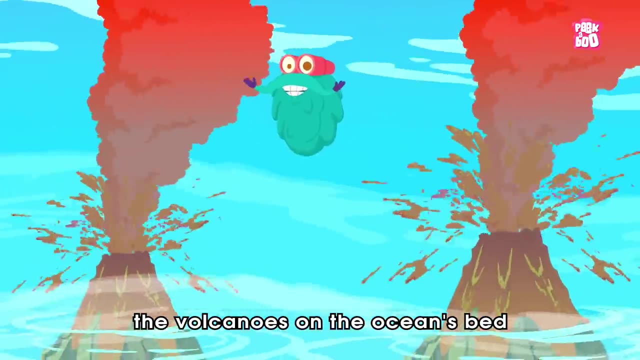 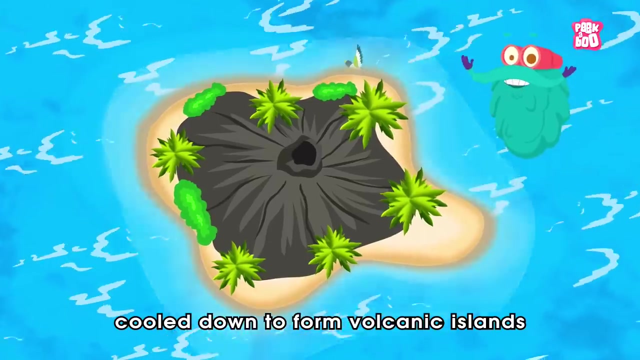 So gradually, the earth cooled down and the surface formed a thin crust. Meanwhile, the volcanoes on the ocean's bed Blew magma to the top, Which eventually cooled down to form volcanic islands That joined together to create a single giant continent called Pangea. 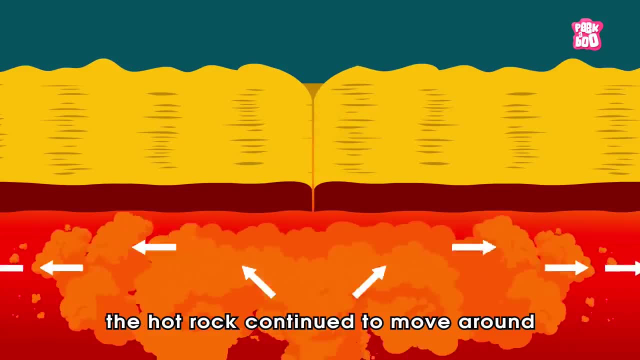 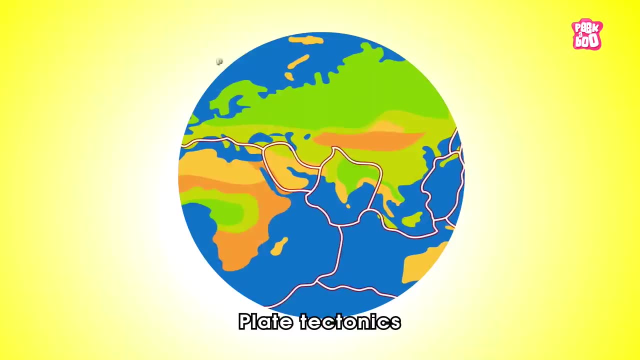 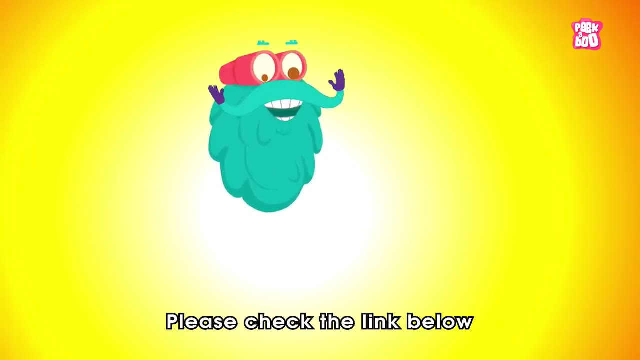 And inside the earth, the hot rock continued to move around, Moving the crust below and breaking it apart Through a process called plate tectonics. We have a separate video dedicated wholly to this topic. Please check the link below. And as the earth's crust moved around,